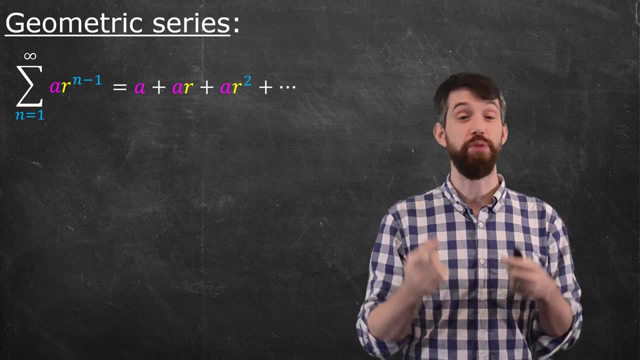 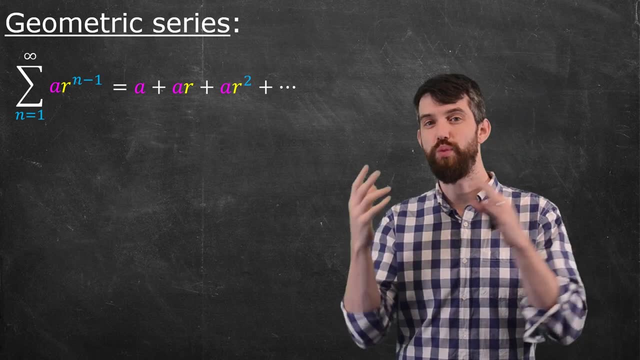 so r to the 0 is 1,, so just a. and then when you plug in n equal to 2,, you get r to the power of 1, so ar and so on. And so far we've seen examples where r was one-half or r was. 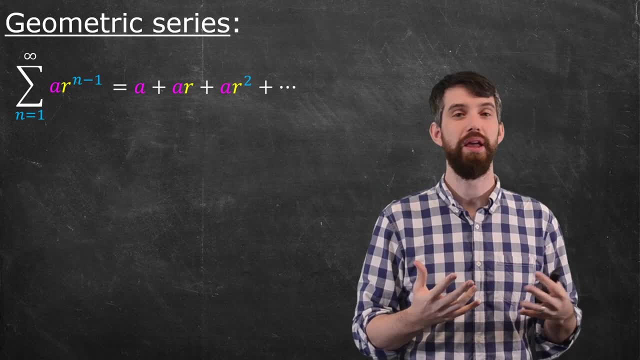 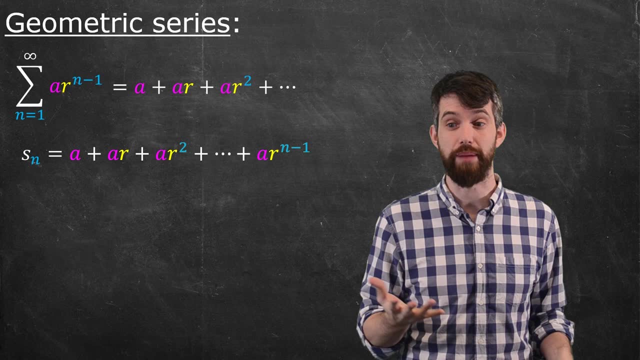 one-third, but we can do this generally for arbitrary r. Now, does this converge? Does this diverge? Does it depend on the parameters? Well, consider this. I want to investigate the partial sum, so let me do this. I'll write down s sub n, the partial sum and the nth. 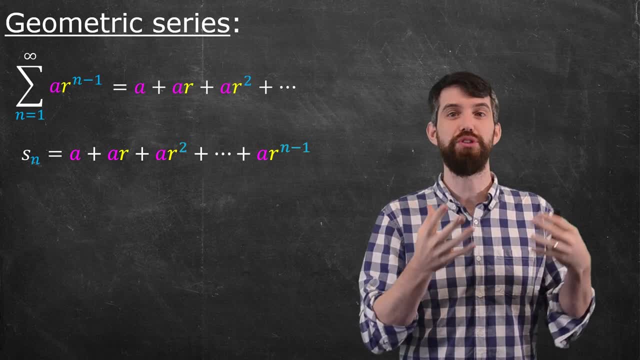 partial sum is the sum of a plus ar, all the way up to ar, to the n minus 1.. Now I'm going to perform a little algebraic trick here. Let me take this n-th partial sum and I'm going to take the n-th partial sum and I'm 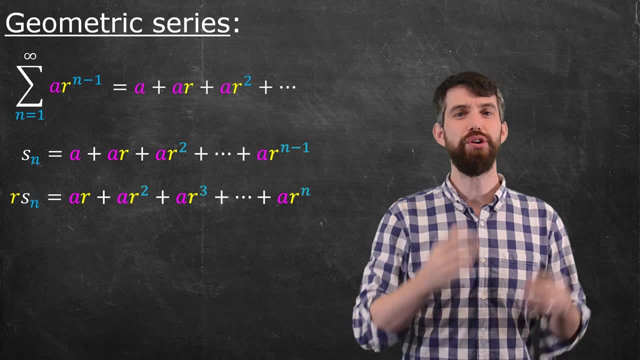 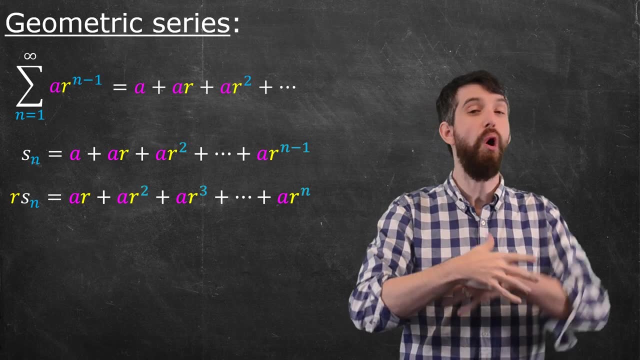 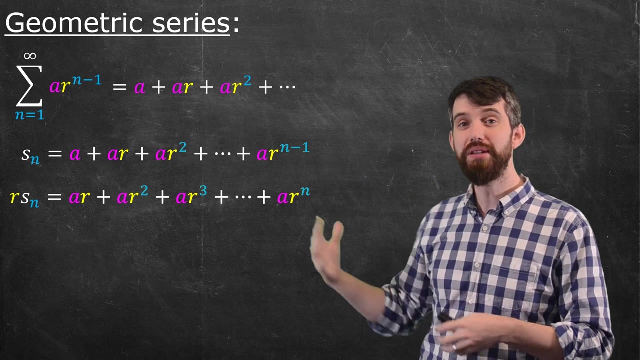 going to take this s-n and let me multiply r to it As in: let me consider r times s-n. So a turns into a times r, a r turns into a times r, squared all the way along. the final one is a r to the n. Now I've got this s-n and I've got r times it, and let me take 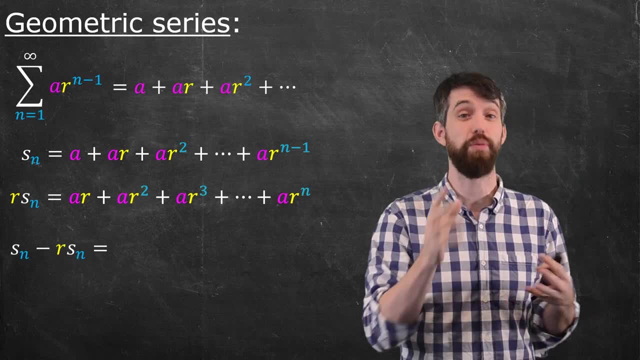 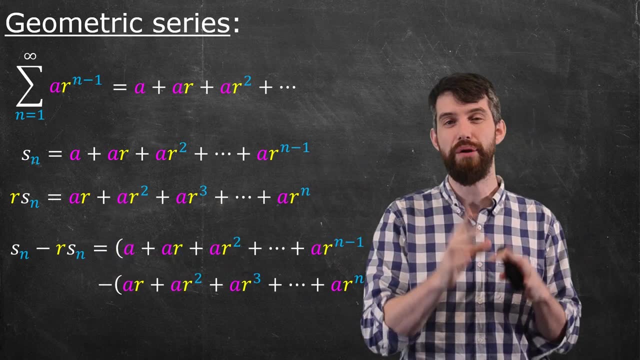 the difference. Let me look at what the partial sum minus r times the partial sum is going to be Indeed. this is plugging in for the s-n that's going to move down. and then I take the r-s-n and I subtract that off. 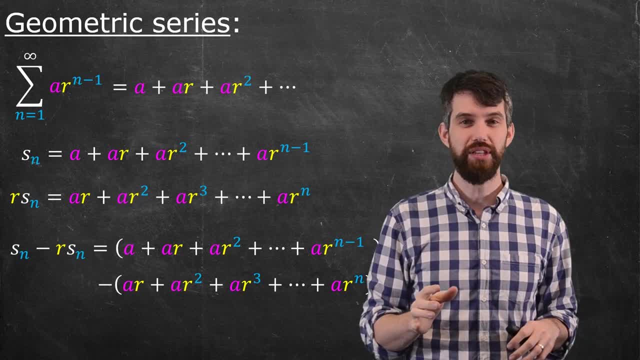 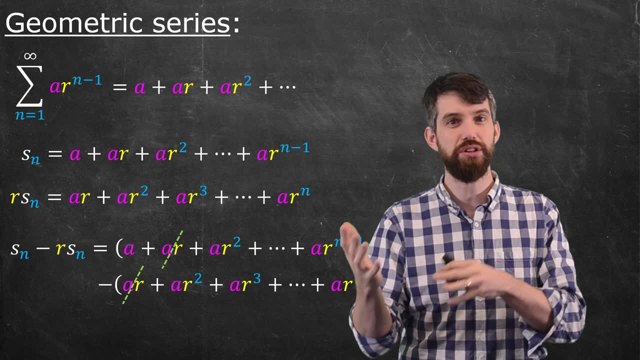 There is an enormous amount of cancellation. For example, you see how that there's a plus ar and a minus ar. Well then, those two terms are just going to cancel. There's a plus ar squared, a minus ar squared. those terms are going to cancel Somewhere in the dot dot. 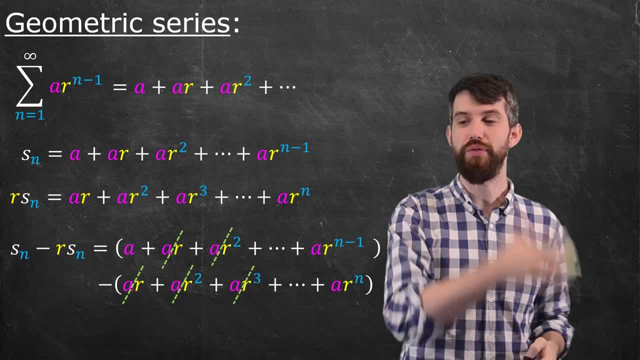 dot, there'd be a positive ar cubed and there's a minus ar cubed, so that cancels. and finally also in the dot dot dot is going to be a subtraction of ar to the n minus 1, that will. 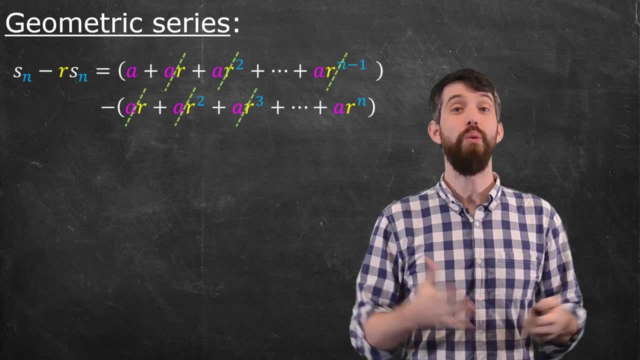 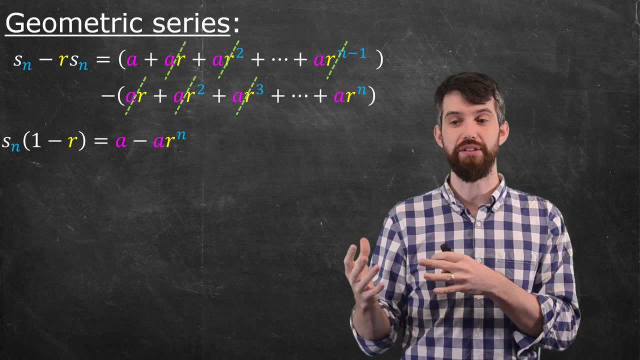 cancel the ar to the n minus 1.. So what do I actually have left Over here? the only thing that remains is going to be the a and the ar to the n. So this difference, which I will factor out the s-n, comes out the front the partial sum. 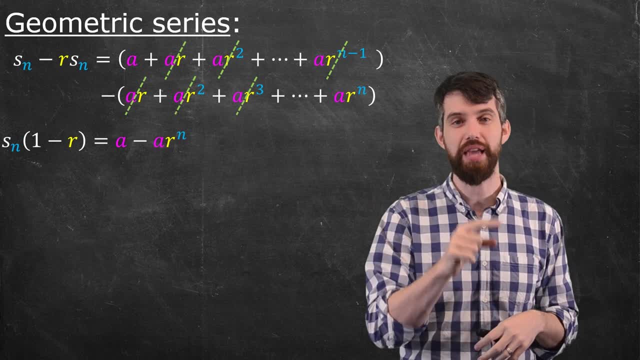 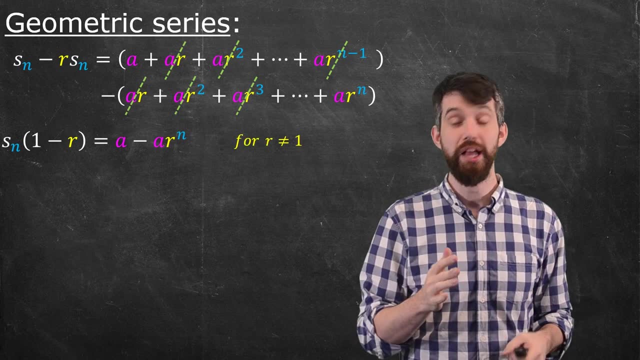 times 1 minus r is just equal to a minus ar to the n. Now if I focus on a special case- this is the case where r is not equal to 1, then I can divide out by 1 minus r and just. 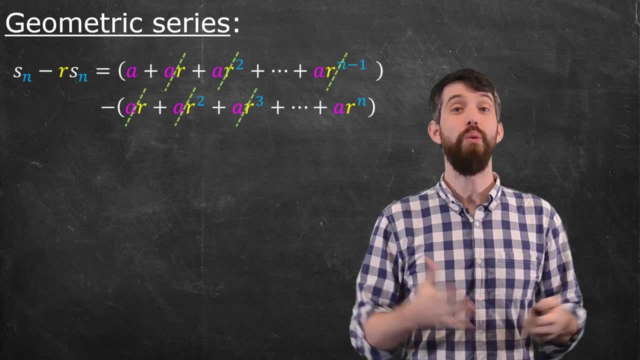 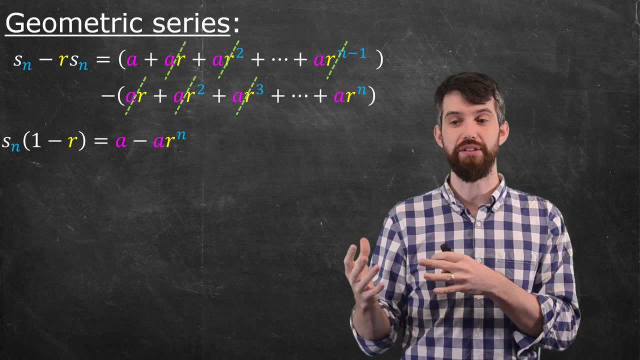 cancel the ar to the n minus 1.. So what do I actually have left Over here? the only thing that remains is going to be the a and the ar to the n. So this difference, which I will factor out the s-n, comes out the front the partial sum. 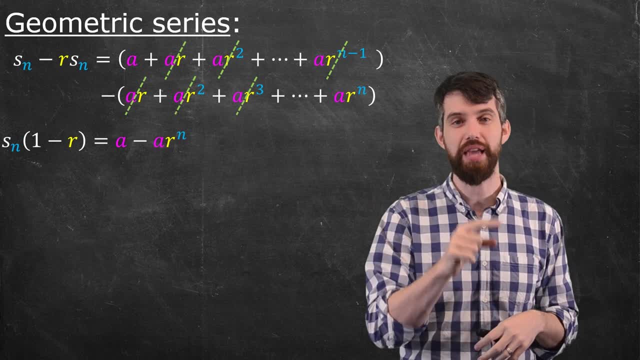 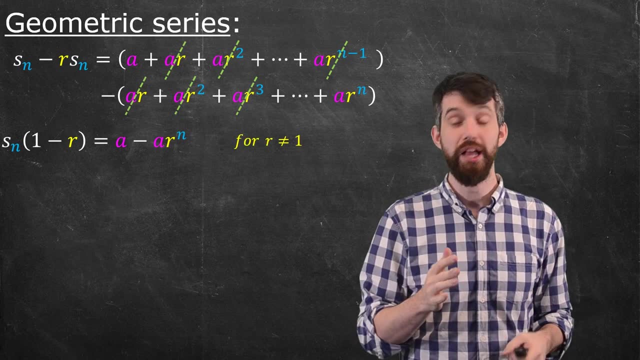 times 1 minus r is just equal to a minus ar to the n. Now if I focus on a special case- this is the case where r is not equal to 1, then I can divide out by 1 minus r and just. 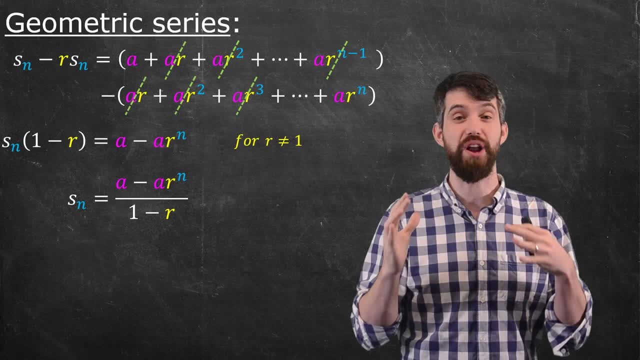 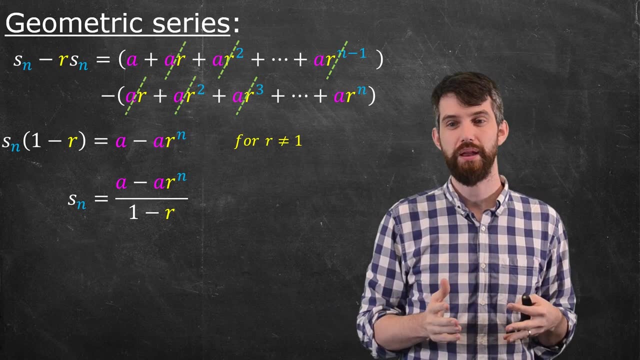 get that. my partial sum is a minus a to the r, divided out by 1 minus r. Of course, if I can't do that, I'll talk about that a little bit more in a moment. Now what I'm investigating is: does this series converge? I'm asking whether the series converges by 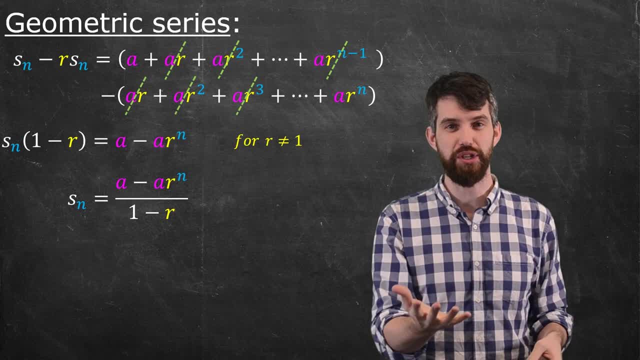 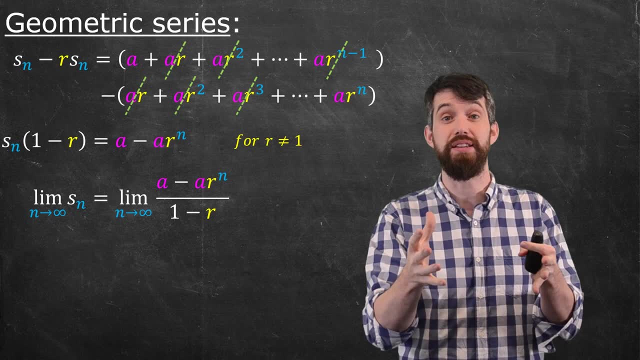 definition meant: does the limit of the partial sums converge? So I have a formula for the partial sums and now I want to ask: well, what about the limit, as n goes to infinity of this sequence of partial sums? So I want to compute this limit. Well, the only way 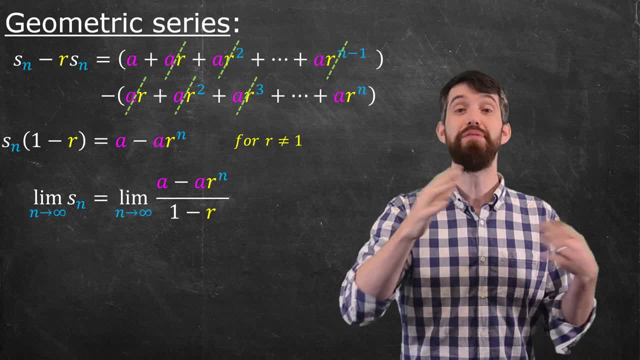 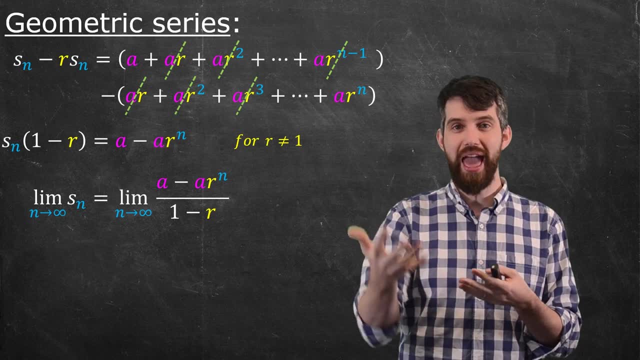 that n appears here is in this r to the n portion. So we have to investigate that Now. imagine r is a number bigger than 1, like, say, 2.. In this case, 2 to the power of n, as n gets large, is going to diverge When r is greater than. 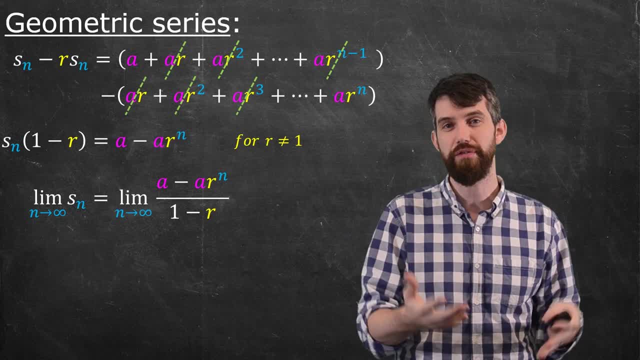 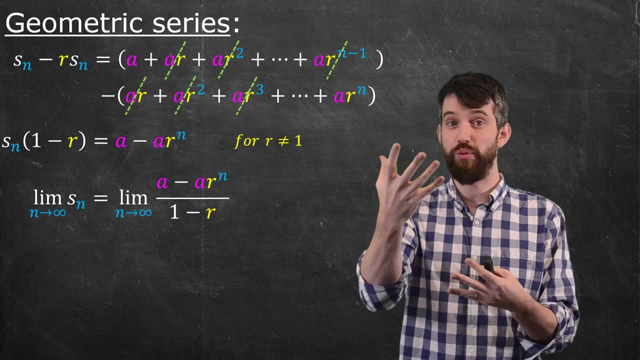 1. here the r to the n term is going to blow up, The whole thing will diverge. But if r is less than 1, say a number like 1 half, 1 half to the power of something really big gets really small. So that portion goes away in the limit. So the point is it depends. 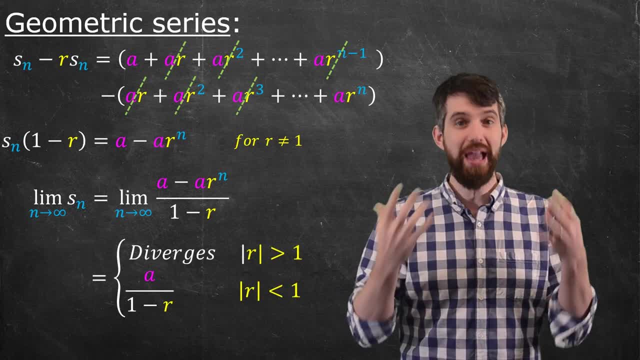 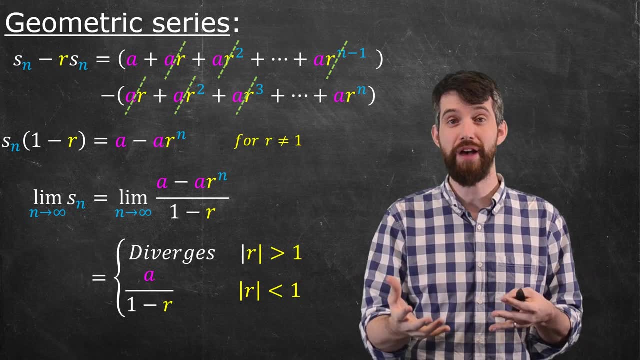 on the value of r. Our final way of saying it is that the magnitude of r- so taking the absolute value here- is greater than 1, then this is going to diverge. It's not going to settle at a value. But if 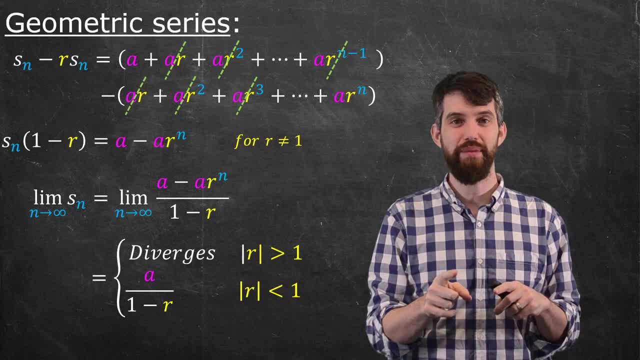 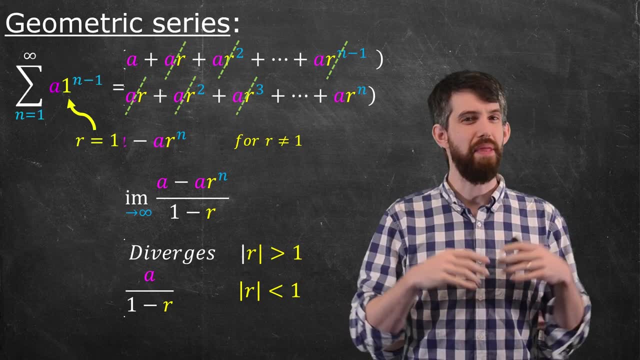 the magnitude of r is less than 1, then that whole term, the r to the n term, is going to go away and I'm just left with an a on the top and a 1 minus r on the bottom. And then I guess the final case I need to analyze is what happens if it's r equal. 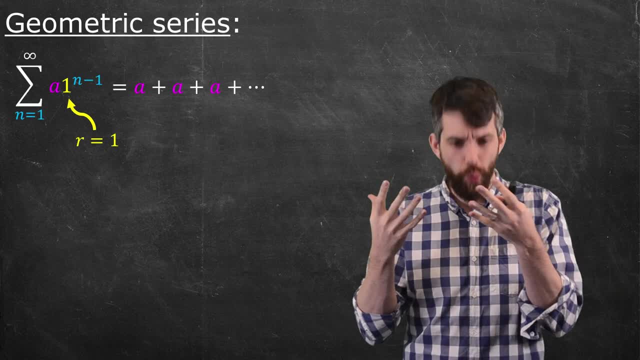 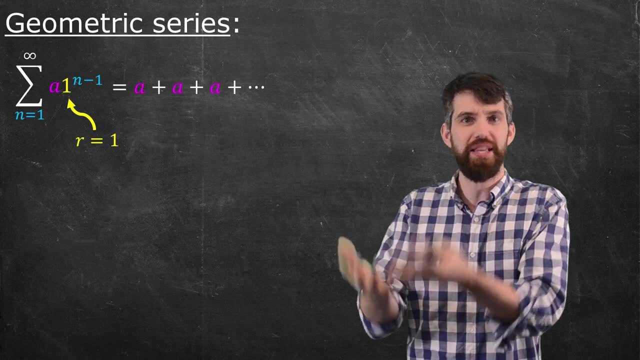 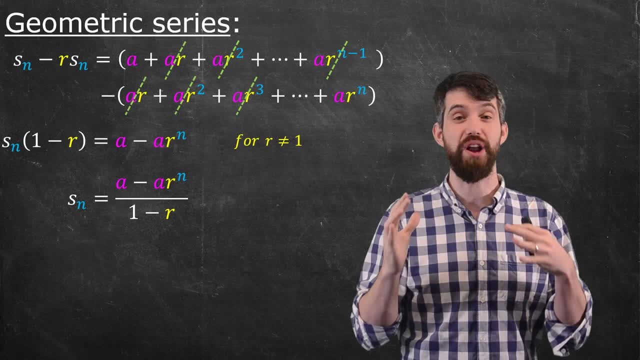 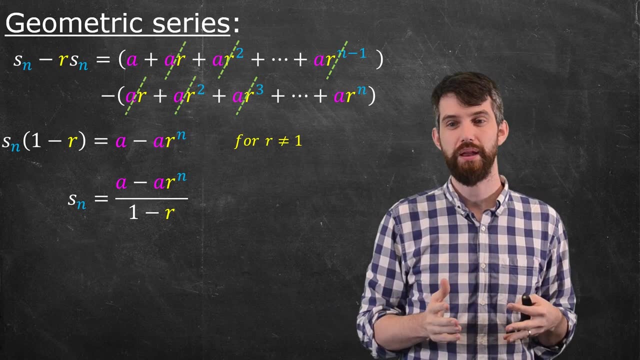 get that. my partial sum is a minus a to the r, divided out by 1 minus r. Of course, if I can't do that, I'll talk about that a little bit more in a moment. Now what I'm investigating is: does this series converge? I'm asking whether the series converges by 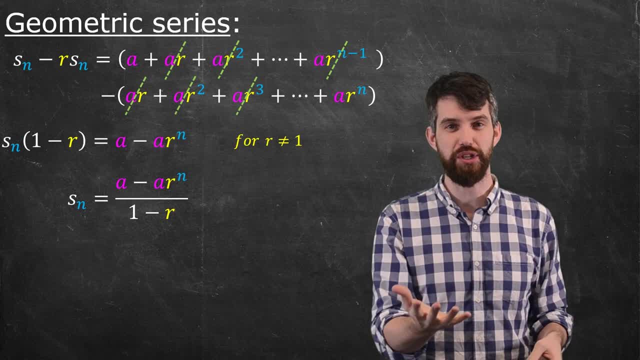 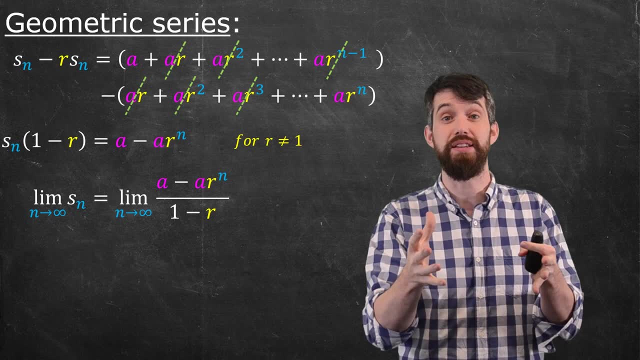 definition meant: does the limit of the partial sums converge? So I have a formula for the partial sums and now I want to ask: well, what about the limit, as n goes to infinity of this sequence of partial sums? So I want to compute this limit. Well, the only way 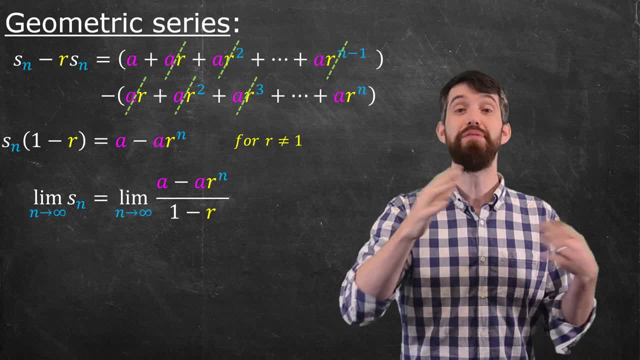 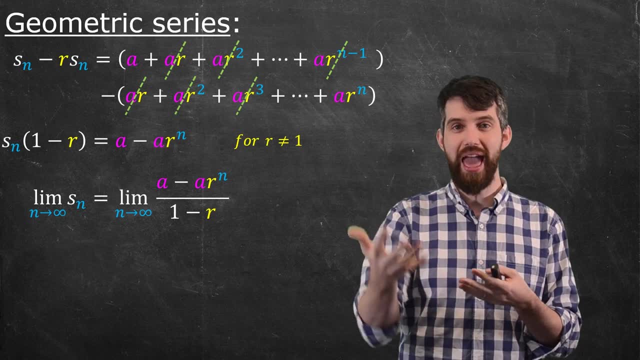 that n appears here is in this r to the n portion. So we have to investigate that Now. imagine r is a number bigger than 1, like, say, 2.. In this case, 2 to the power of n, as n gets large, is going to diverge When r is greater than. 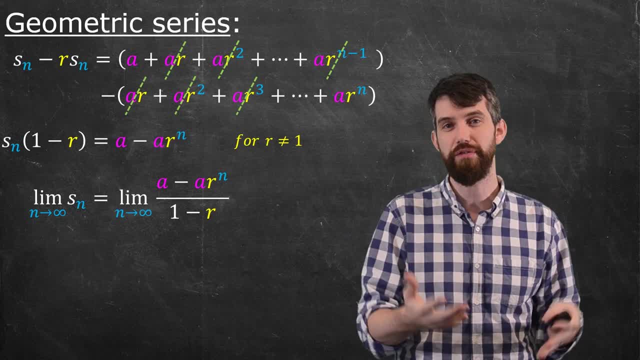 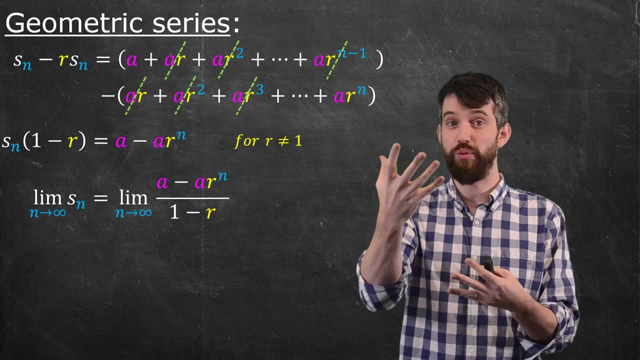 1. here the r to the n term is going to blow up, The whole thing will diverge. But if r is less than 1, say a number like 1 half, 1 half to the power of something really big gets really small. So that portion goes away in the limit. So the point is it depends. 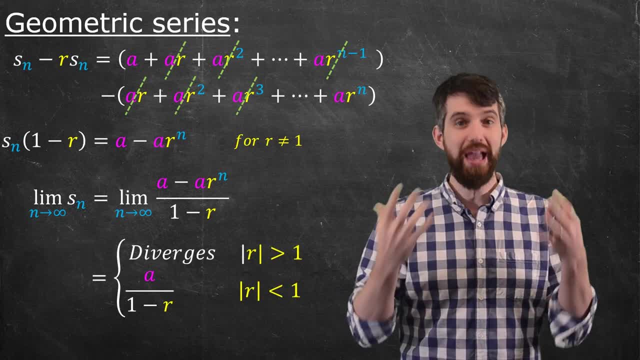 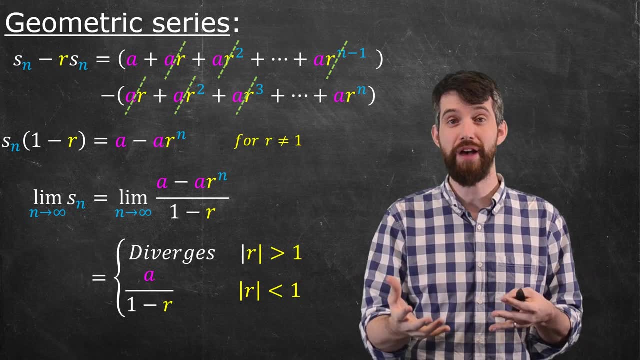 on the value of r. Our final way of saying it is that the magnitude of r- so taking the absolute value here- is greater than 1, then this is going to diverge. It's not going to settle at a value. But if 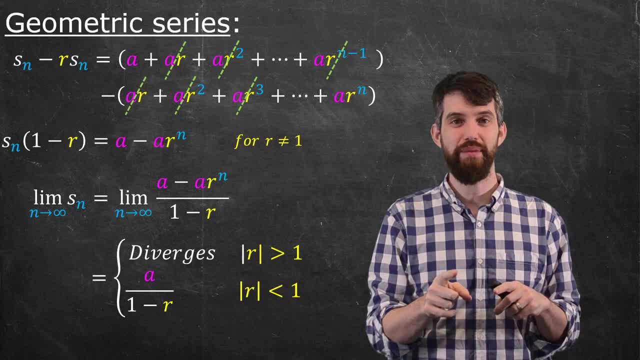 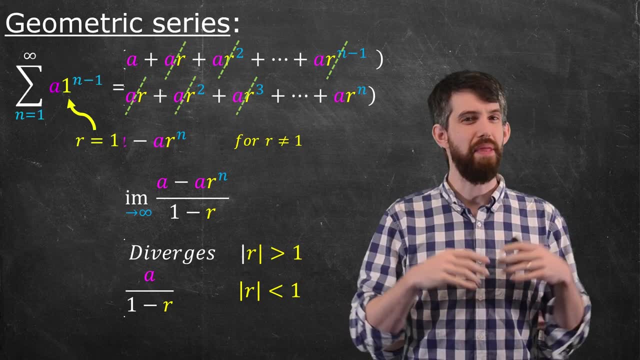 the magnitude of r is less than 1, then that whole term, the r to the n term, is going to go away and I'm just left with an a on the top and a 1 minus r on the bottom. And then I guess the final case I need to analyze is what happens if it's r equal. 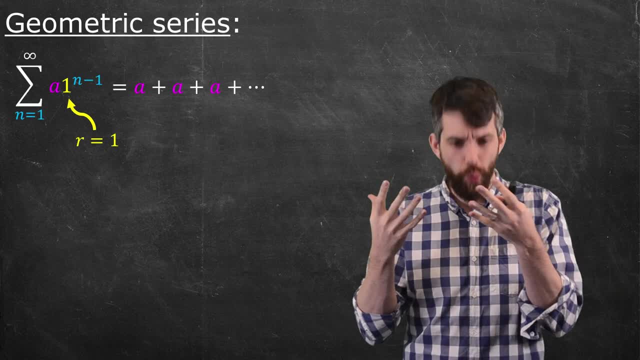 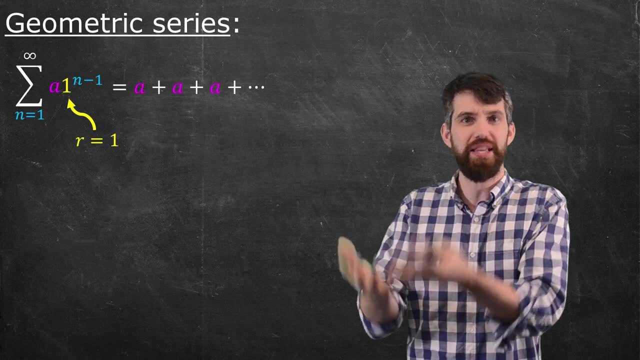 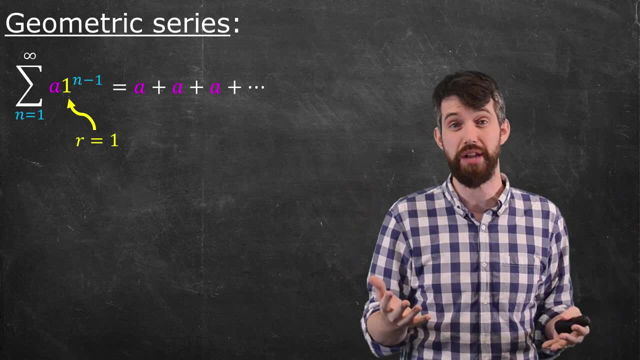 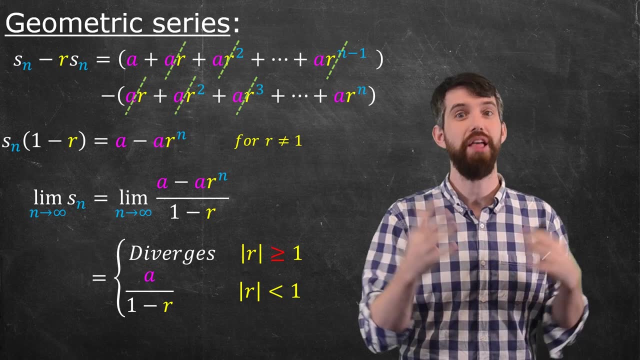 sum, which is taking the constant and adding it up, is clearly going to diverge. So, indeed, I can replace this with not just greater than 1, but greater than or equal to 1.. That's when it's going to diverge. So for the geometric series, we know exactly when it converges. 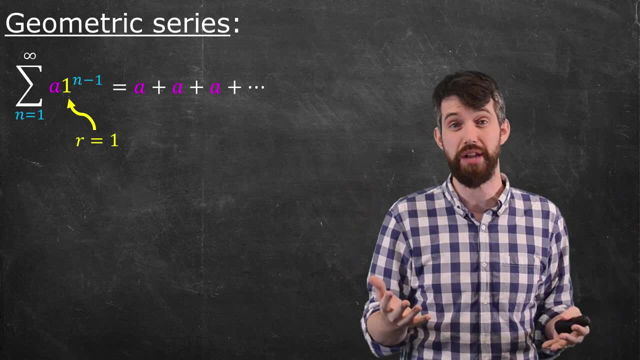 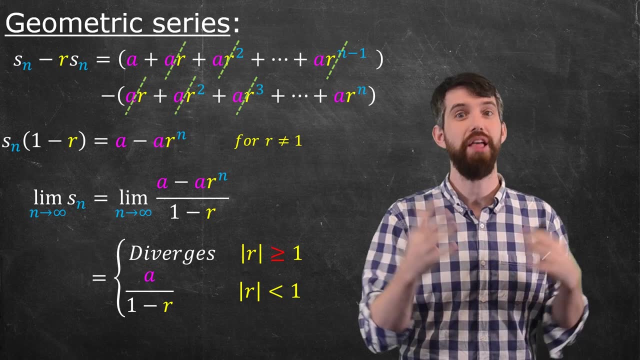 sum, which is taking the constant and adding it up, is clearly going to diverge. So, indeed, I can replace this with not just greater than 1, but greater than or equal to 1.. That's when it's going to diverge. So for the geometric series, we know exactly when it converges. 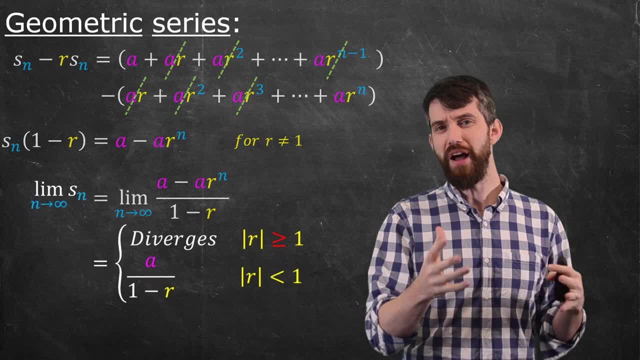 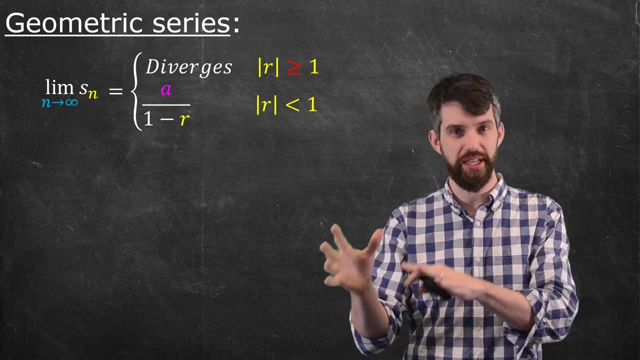 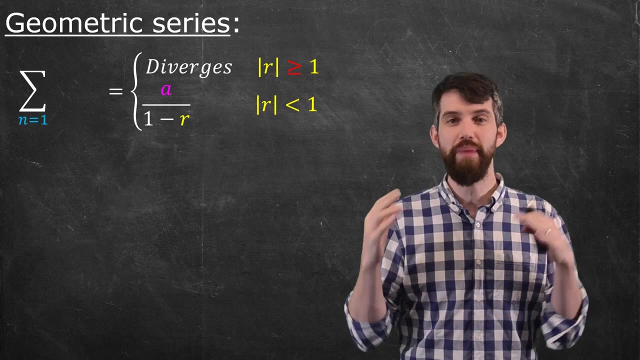 and exactly when it diverges. And then, finally, this is just the limit of the partial sums, That if the limit of the partial sums converges, then so too does the series. That is how we define convergence of a series. So then I can say that the summation of this ar to 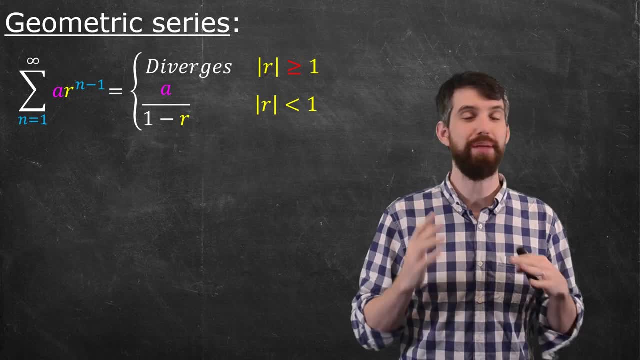 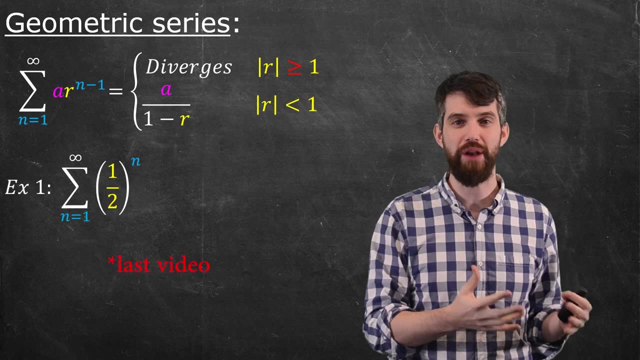 the power of n minus 1, that that diverges for the absolute value of r bigger or equal to 1 and converges for less than 1.. Let's see this for the examples we began with For the particular series, that's adding 1, half, 1 quarter, 1 eighth and so on. this is just. 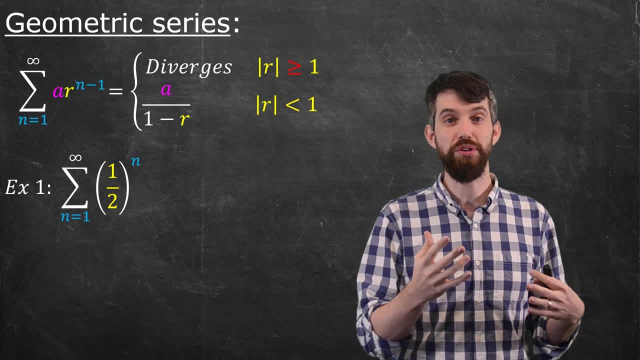 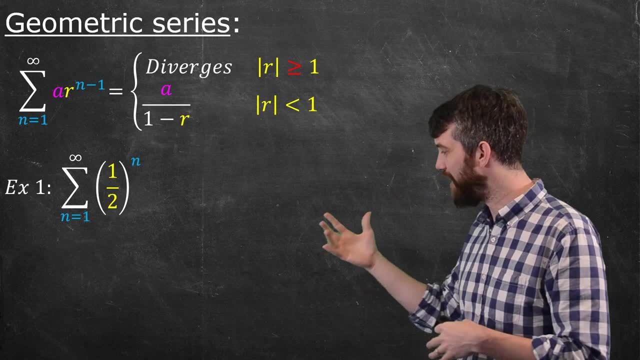 1, half to the power of n. Now this is almost of the format of the geometric series, but notice, the indexing here is not to the power of n minus 1, it's to the power of n here. So why don't I just pull out a? 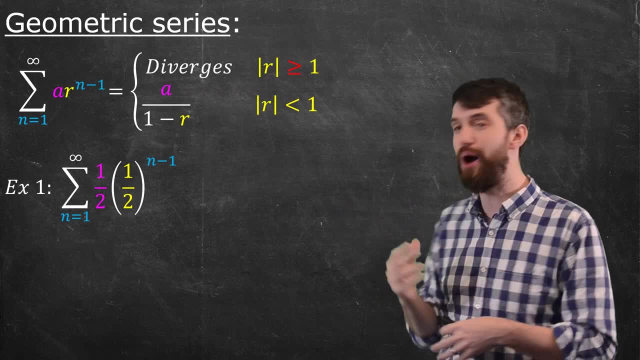 factor of 1 half. I'll put that into the constant. and now it's to the power of n minus 1.. So I've sort of aligned my formulas here. My a is 1 half, and now I've got to the power. 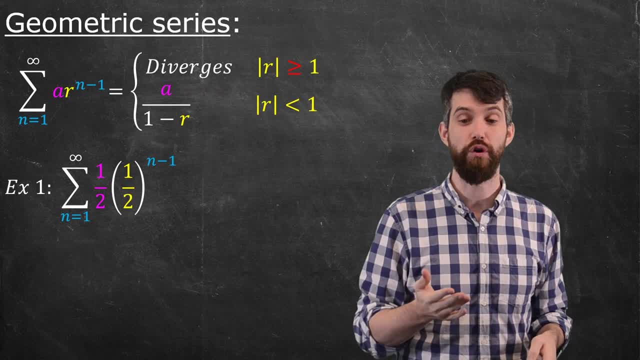 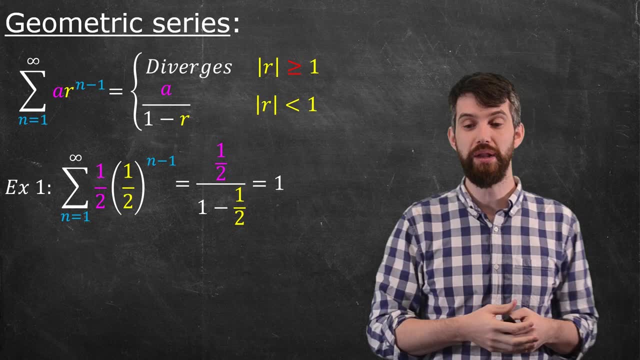 of n minus 1 on my other 1 half. Okay, plug in my formula here r is less than 1, so it's in the convergence case 1 half is less than 1. And indeed it equals 1.. So indeed, if I want to go one unit away and I go half the 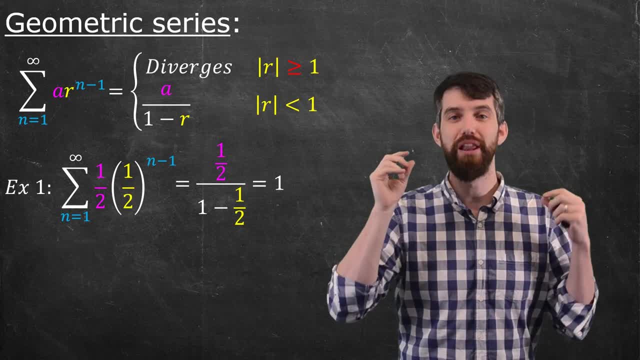 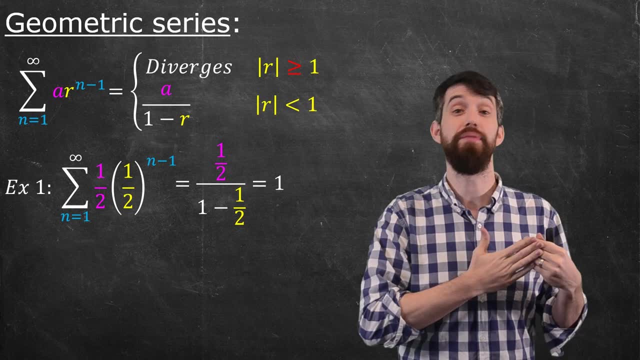 distance, then a quarter, then the eighth and the sixteenth. I add all of those up, I will eventually get at least in the limit- as these things are going to infinity, converging to the value of 1, to have gone the entire way across this length. But if it was only 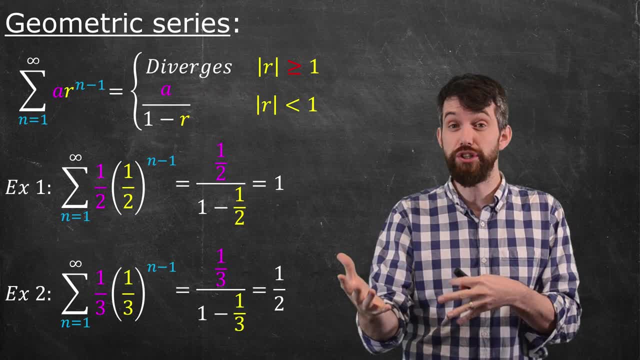 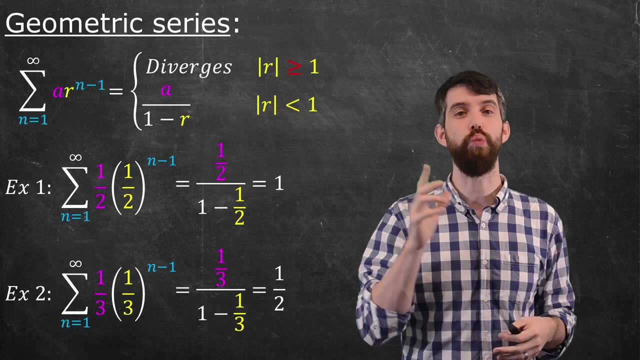 1 third, it still converges. It still converges because the r is less than 1, the 1 third is less than 1.. Now, when I look at its sum, it adds up to 1 half. So going: 1 third, 1 ninth, 1 twenty-seventh. 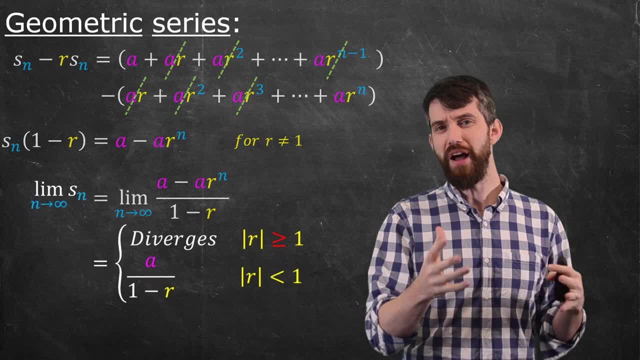 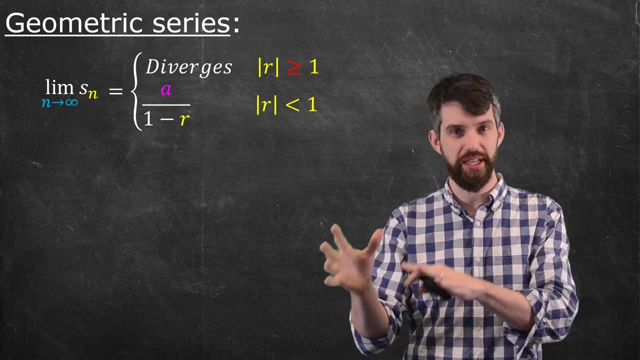 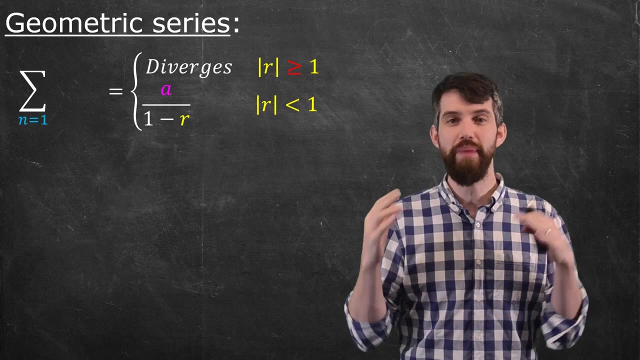 and exactly when it diverges. And then, finally, this is just the limit of the partial sums, That if the limit of the partial sums converges, then so too does the series. That is how we define convergence of a series. So then I can say that the summation of this ar to 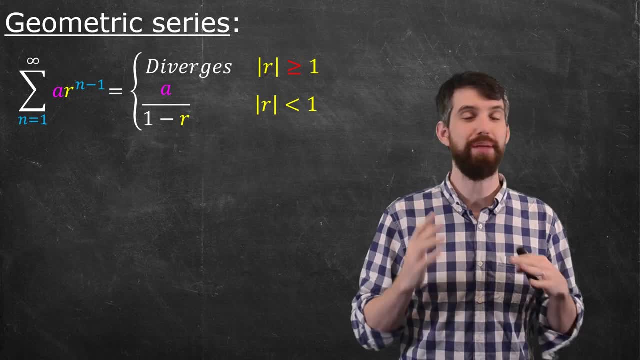 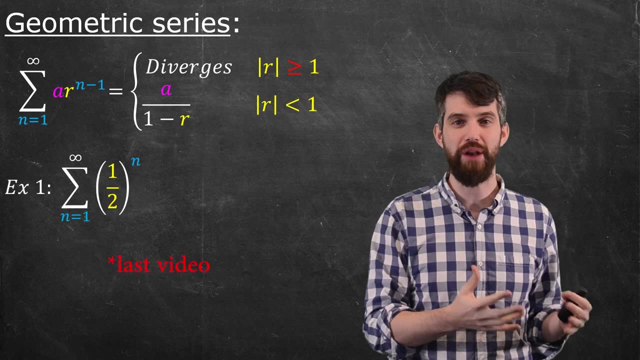 the power of n minus 1, that that diverges for the absolute value of r bigger or equal to 1 and converges for less than 1.. Let's see this for the examples we began with For the particular series, that's adding 1, half, 1 quarter, 1 eighth and so on. this is just. 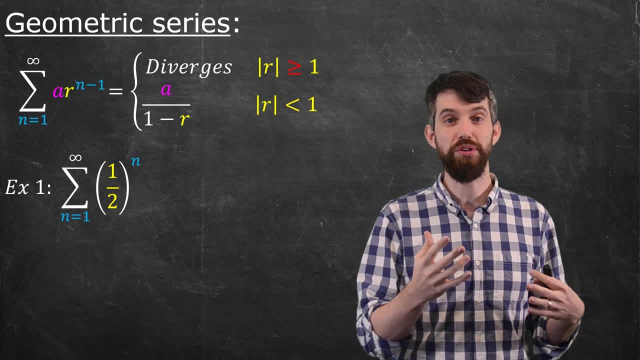 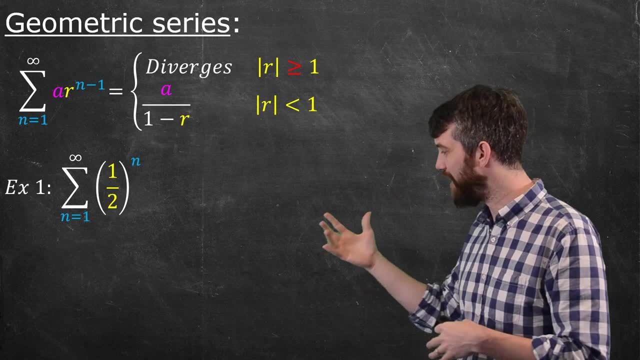 1, half to the power of n. Now this is almost of the format of the geometric series, but notice, the indexing here is not to the power of n minus 1, it's to the power of n here. So why don't I just pull out a? 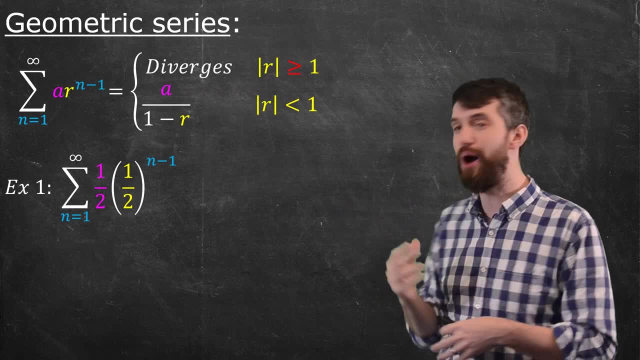 factor of 1 half. I'll put that into the constant. and now it's to the power of n minus 1.. So I've sort of aligned my formulas here. My a is 1 half, and now I've got to the power. 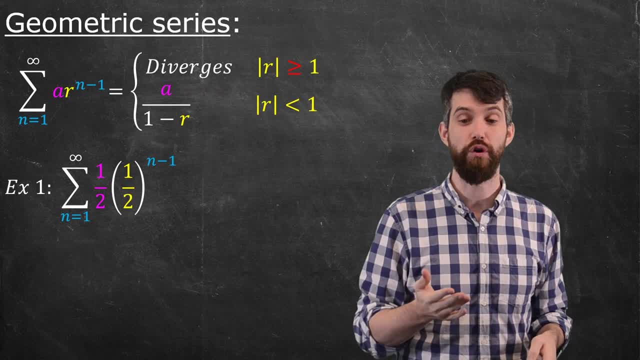 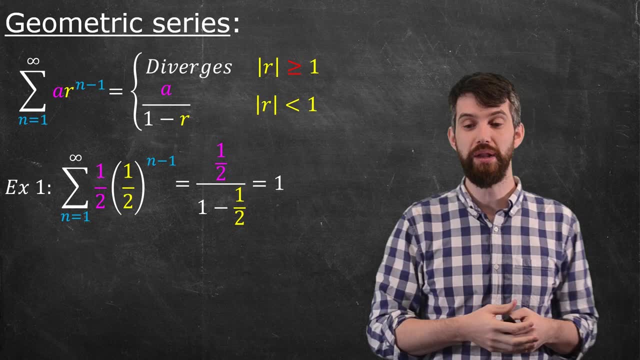 of n minus 1 on my other 1 half. Okay, plug in my formula here R is less than 1, so it's in the convergence case 1 half is less than 1. And indeed it equals 1.. So indeed, if I want to go one unit away and I go half the 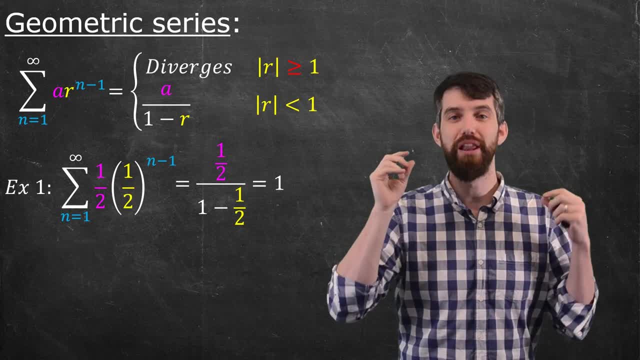 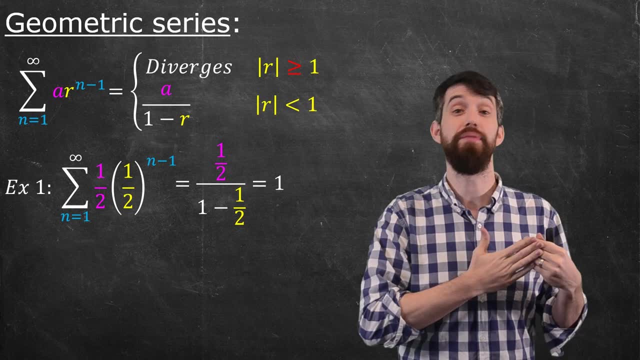 distance, then a quarter, then the eighth and the sixteenth. I add all of those up, I will eventually get at least in the limit- as these things are going to infinity, converging to the value of 1, to have gone the entire way across this length. But if it was only 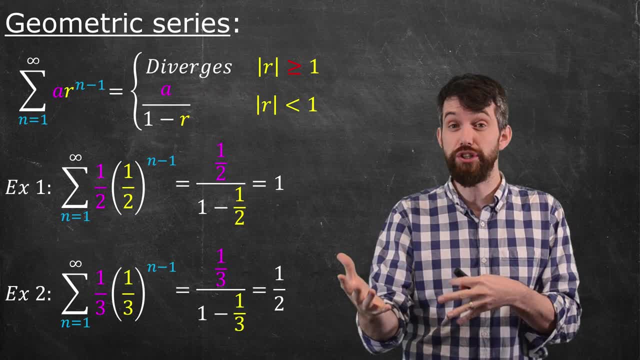 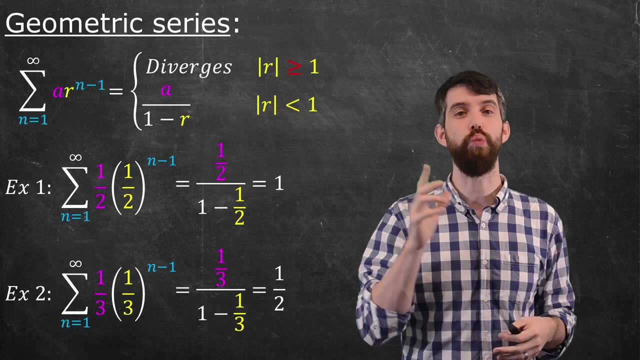 1 third, it still converges. It still converges because the r is less than 1, the 1 third is less than 1.. Now, when I look at its sum, it adds up to 1 half. So going: 1 third, 1 ninth, 1 twenty-seventh. 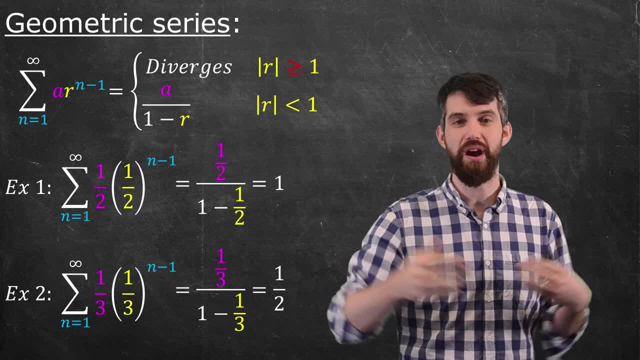 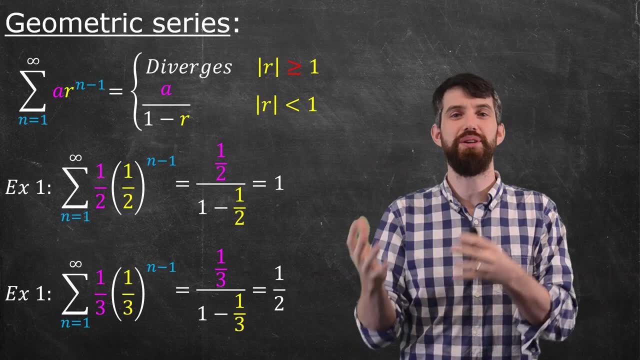 and so on. I'll never get 100% of the way there. I'll never get that one unit away. I'll only get half of the unit away. So in this video we have talked about the geometric series as a special case of the. 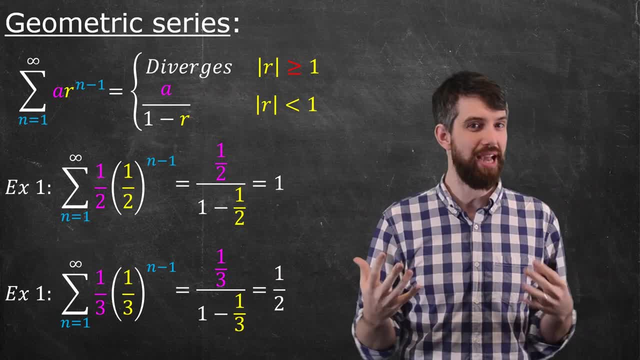 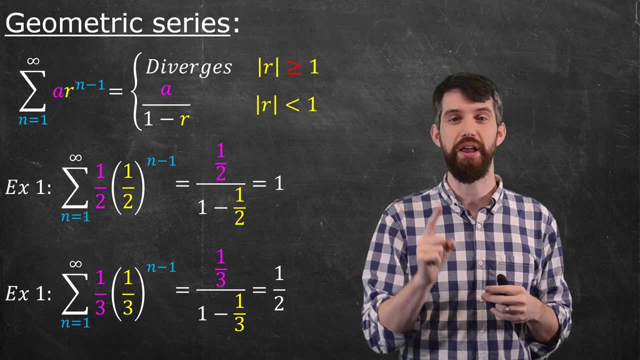 idea of convergence of series, And indeed geometric series are very nice. They're one of the few series where not only can we tell whether it converges or diverges, but we can say exactly what it is, And it converges too.